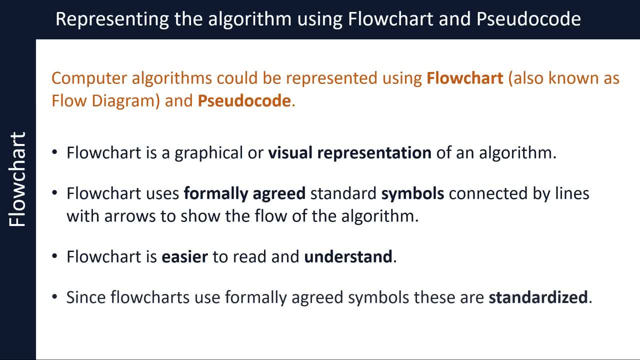 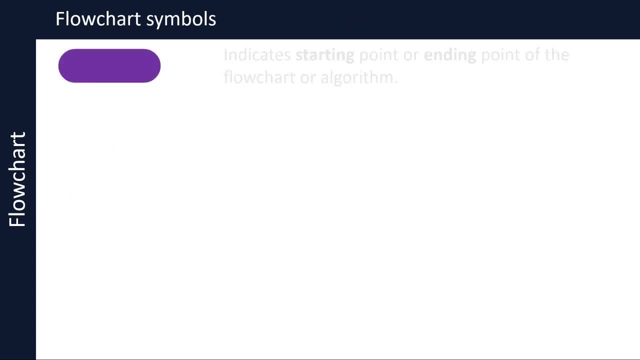 any variations in terms of how flowcharts are presented. Let's now look at symbols used in flowchart. This symbol is used to indicate the start or end of the flowchart. Flowcharts always have starting and ending points in between. This symbol is used to indicate the start. 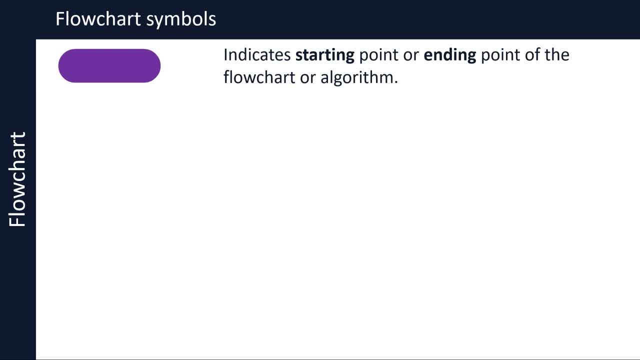 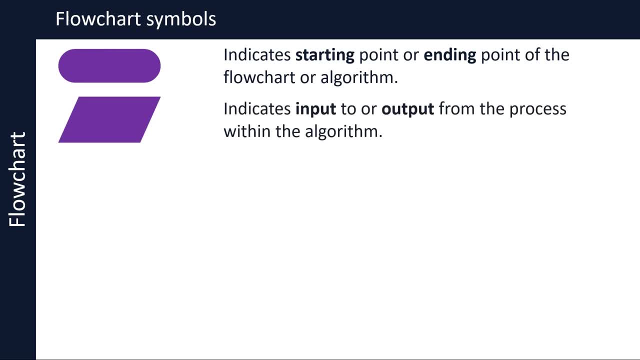 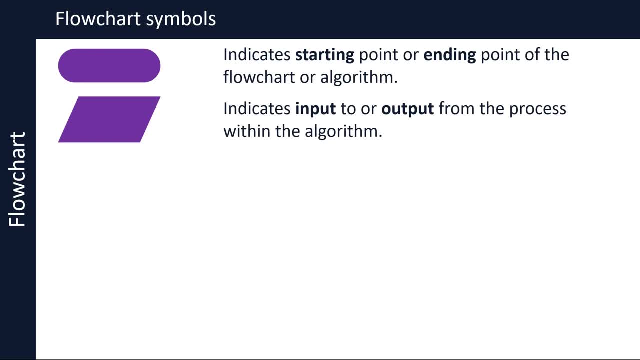 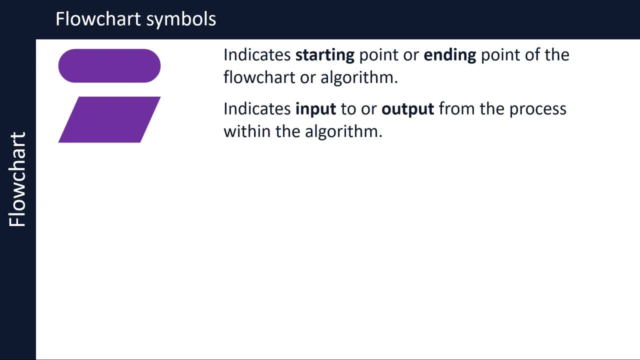 This symbol is used to indicate the start and ending points in between. This symbol is used to indicate the start and ending points in between outputs from the process or operation that is carried out within the algorithm. This symbol is used to indicate the process or operation that is performed within the algorithm. 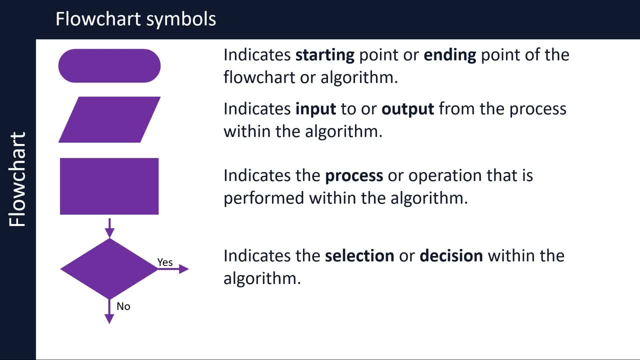 This symbol is used to indicate the selection or decision within the algorithm. It is used to present a question in the algorithm which has only two answers, typically true or false, or yes or no type of answers. Then, depending on the answer, algorithm takes one of the two paths. It always has one arrow going in and two arrows coming out. 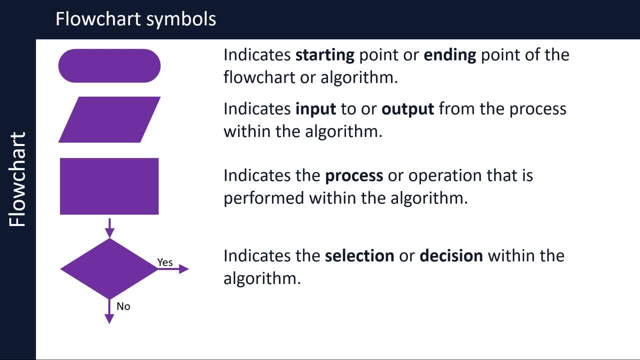 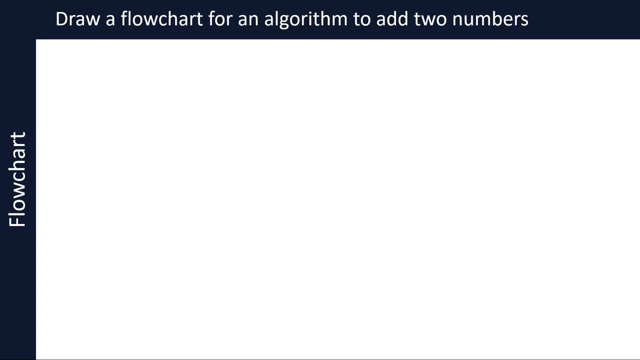 from it showing the two logical paths. The two answers are labeled along the two arrows coming out. One directional arrows link the above symbols showing the logical flow of the algorithm. Let's take an example. Let's use an example of the algorithm to add two numbers that we saw in algorithm's video. 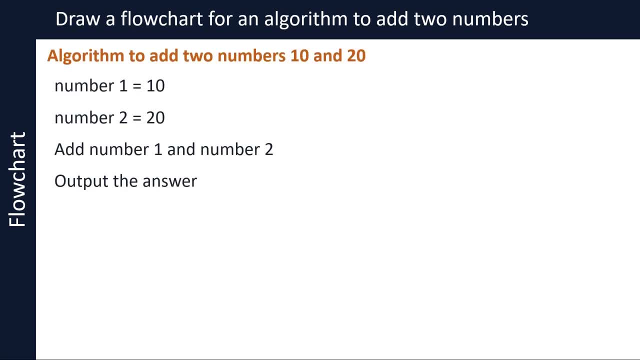 Here is the descriptive text. Set number 1 to 10.. Set number 2 to 20.. Add number 1 and number 2.. Output the answer. Let's now draw the flow chart or flow diagram for this algorithm. This is first symbol for our flow chart, As seen earlier. it denotes the start of the flow chart. 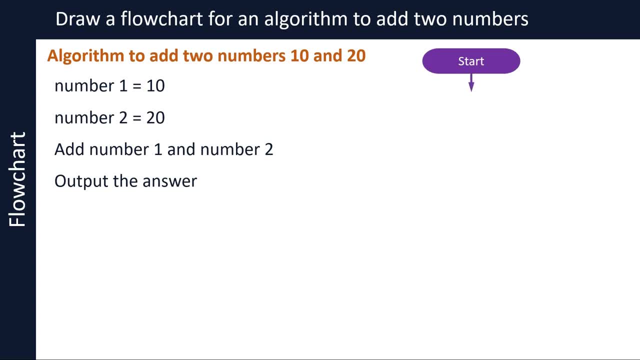 The arrow goes to the first symbol of the flow chart. The arrow coming out from this symbol shows the direction of flow. in the algorithm. We draw the next symbol to denote the process. Here we are assigning the value 10 to number 1.. 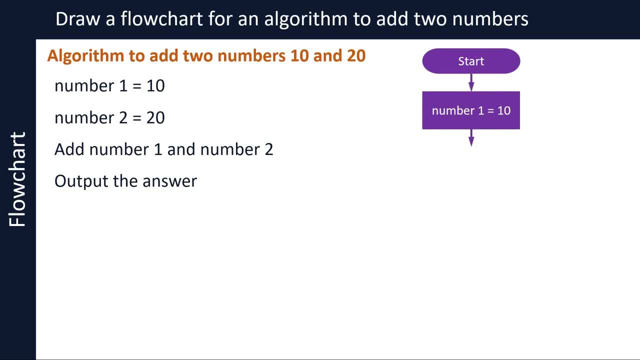 We are using assignment operator or symbol equal to to perform the assignment operation. In computer terminology, number 1 is called variable. We will discuss about variables in detail in a separate video, but let's just talk a little bit about variables before we move further. 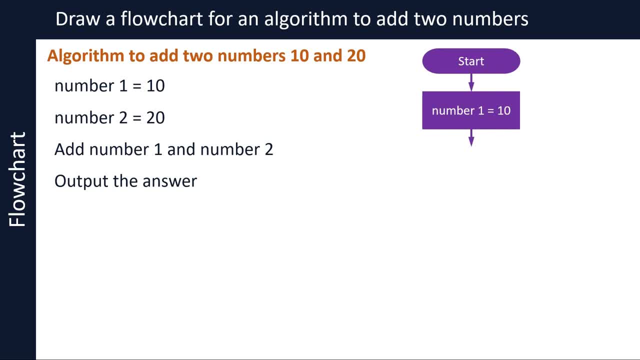 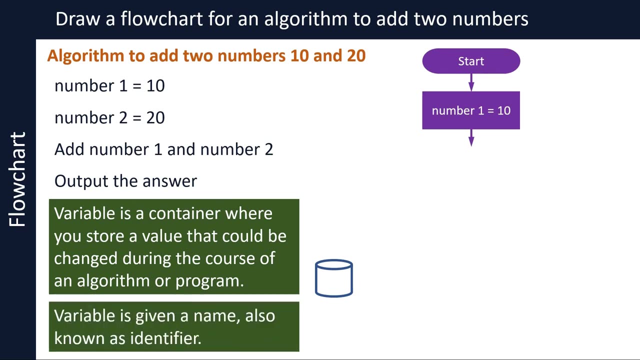 As the name suggests, variable is something that does not have a fixed value. It is a container where you can store a value which could be changed during the course of the algorithm or program. Variable is given a name to so that we can reference a variable by its name. 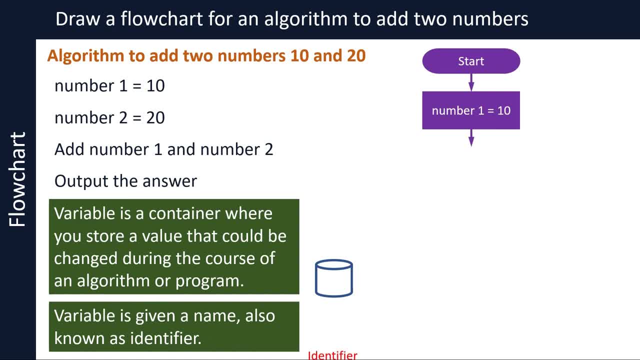 The name of the variable is also known as an identifier. What we are doing here is storing value 10 in a variable called number 1.. We now know that the variable is a variable. We now know that the variable is a variable. We now know that the variable is a variable. 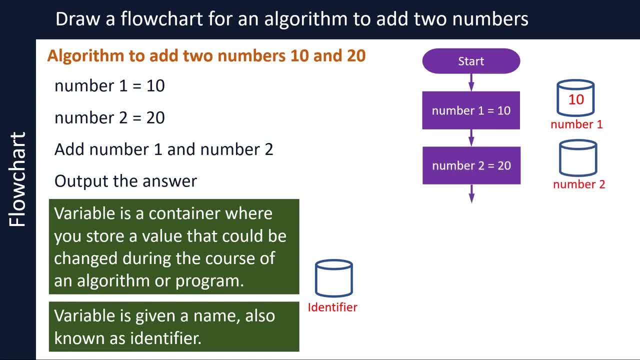 This is a variable. This is a variable. draw process symbol again to denote another process. Here we are assigning value 20 to a variable called number 2.. Or in other words, we are storing value 20 in a variable called number 2.. We draw the next symbol to denote process one more time. Here we are performing. 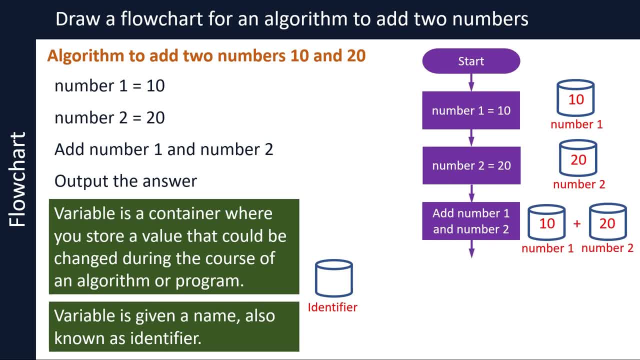 addition operation. So when we say add number 1 and number 2, values stored in variables- number 1 and number 2- will be added together, That is, 10 and 20 will be added together. So whenever we perform any operation on variables in this way, we are instructing computers. 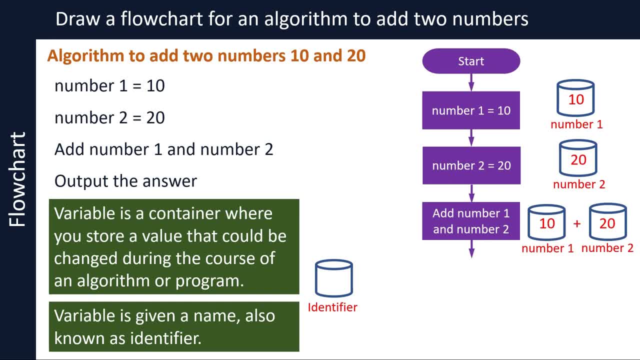 to perform the operation on the values stored in the variables, rather than variable names. This is very similar to the concept of substituting values in the mathematical equation. For example, if you have to solve the equation a plus b and you have been given values as a equals 2 and b equals 5,, then substituting these. 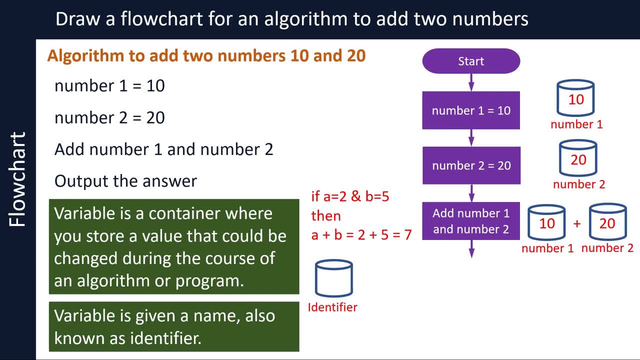 values in the equation. a plus b will become 2 plus 5, which equals 7.. I hope you got the point. We draw our next symbol to denote output. Here we output the answer of adding 10 and 20.. Finally, the last symbol denotes the end of the flowchart. We have drawn our first flowchart. 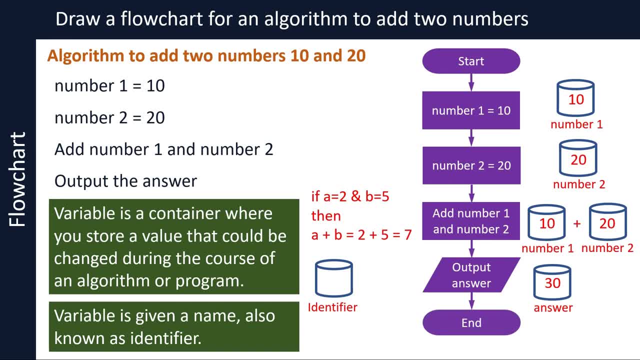 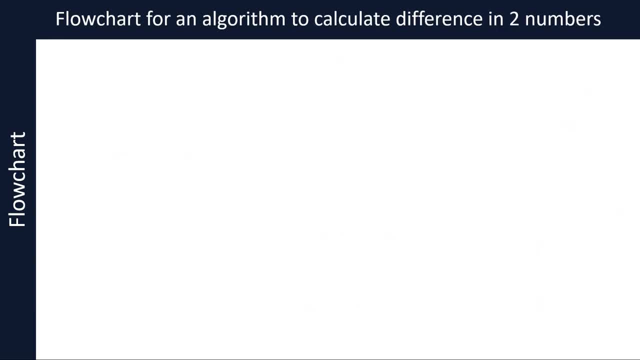 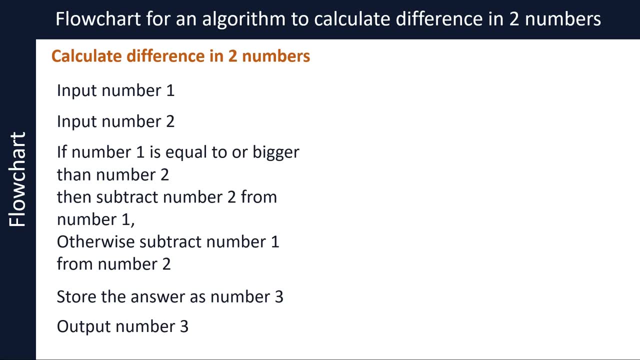 Since this was a very simple algorithm, we did not need to use all the flowchart symbols that we have seen earlier. Let's now look at algorithm to calculate difference in two numbers and draw a flowchart for it. Here is the descriptive text for this algorithm. 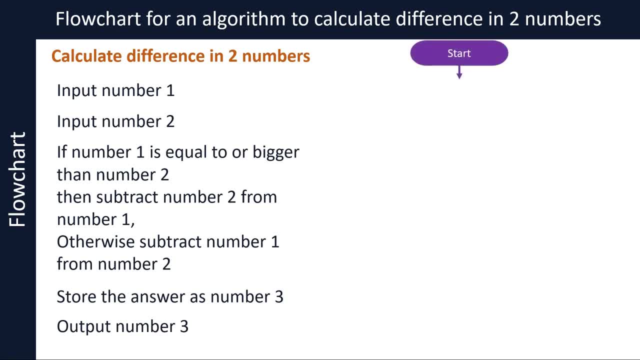 The first symbol denotes the start of the flowchart. The next symbol denotes input that will be used in the process within the algorithm. In this step we are getting user to input the first number and storing that in variable called number 1.. The next symbol denotes another. 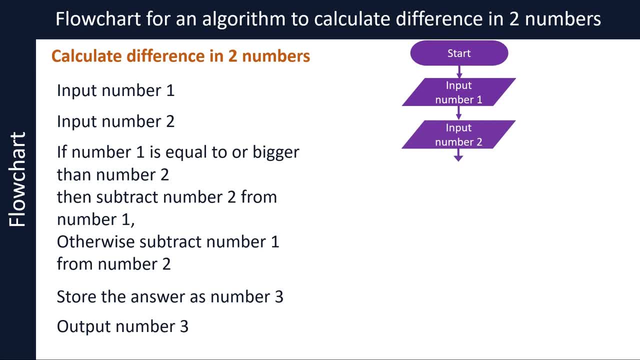 input from user and we are storing that in variable called number 2.. The next symbol is the decision symbol that we have seen earlier but have not used it so far. It denotes decision or selection. Here we are asking a question and making a decision. Is number 1 equal to? 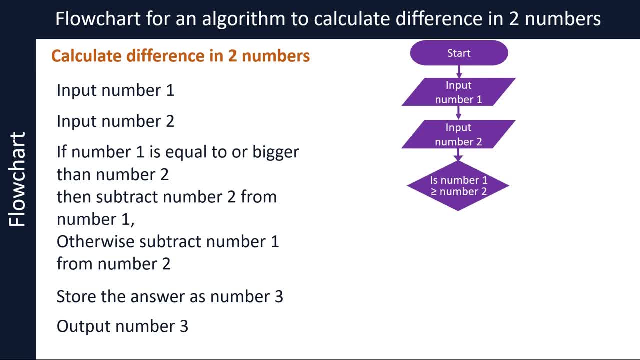 or bigger than number 2?? Here we are using a relational operator greater than or equal to to check if number 1 is equal to or bigger than number 2.. We will talk about various arithmetic, relational and boolean operators in a separate video. 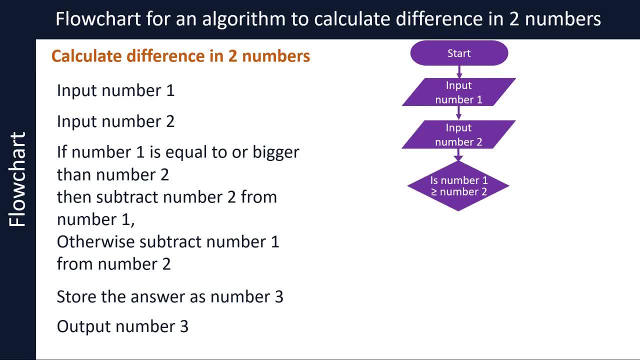 In this step, we are instructing the computer to perform a comparison operation on the value stored in variables rather than variable names, similar to what we saw in previous algorithm. If the answer is yes, that is, if number 1 is equal to or bigger than number 2, then 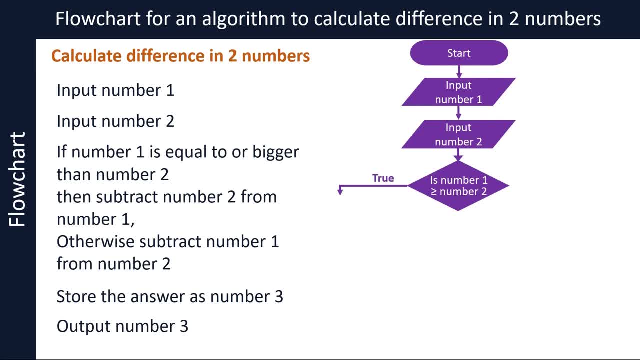 we will take the path along the arrow labelled with true. If answer is no, then we will take the path along the arrow labelled with false. We now draw a process symbol along the true path to denote a process where we subtract number 2 from number 1, that is Subtract. 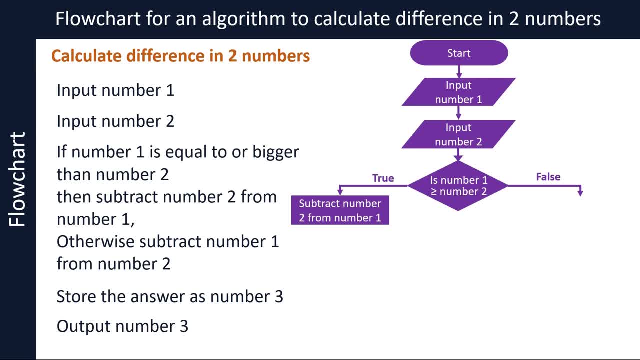 the value stored in variable number 2 from the value stored in variable number 1.. We now draw a process symbol along the false path to denote a process where we subtract value stored in variable number 1 from value stored in variable number 2.. You need to understand. 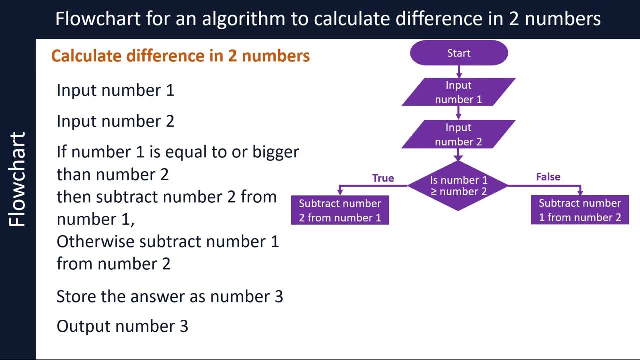 that at any given path through the algorithm, computer will only take one of the two routes: A route along the true path if the number 1 is equal to or greater than number 2, or route along the false path. otherwise, These both paths will lead to the next step. The next symbol is process. again, It shows: 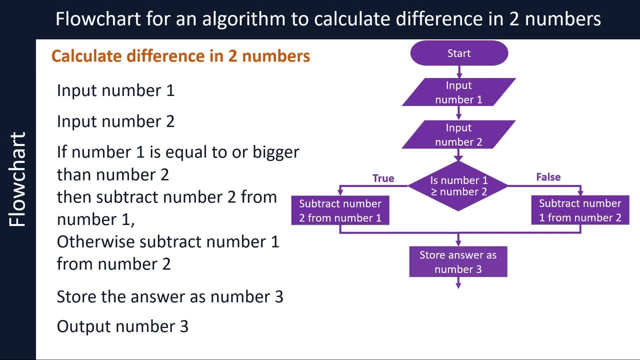 the process of storing the result of one of the two subtraction operations performed earlier in a third variable called number 3.. As you can see paths from both the subtraction operation leads to the process of storing the result into a third variable called number 3.. The 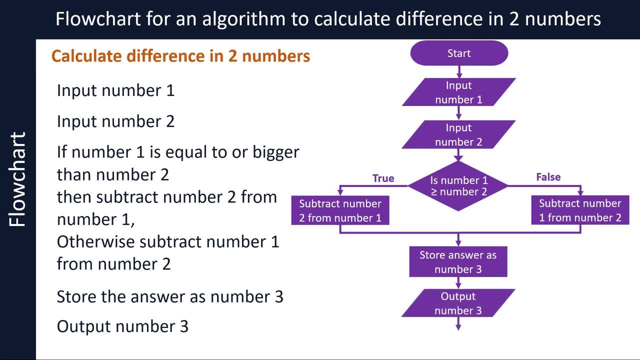 next symbol denotes output. Here we output the results to the second variable. It is the value stored in variable number 3.. It is the value stored in the variable that will be output here, rather than the variable name. Finally, symbol denotes the end of the flow chart. Single directional arrows in the flow. 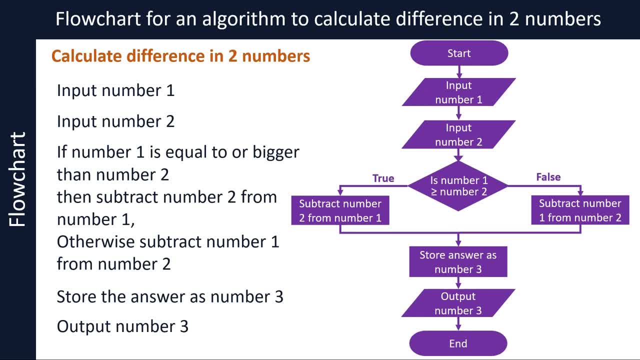 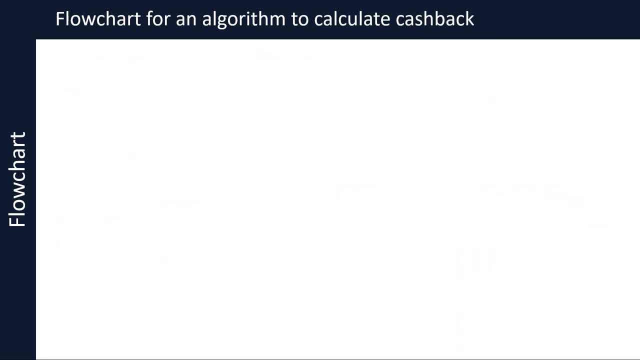 chart shows the direction of flow in the algorithm. Let's now take one final example before we conclude this topic. A bank has launched a new credit card and they are offering 5% cash back on purchases over $500.. The bank is charging the bank cash back in the first month as an introductory offer. 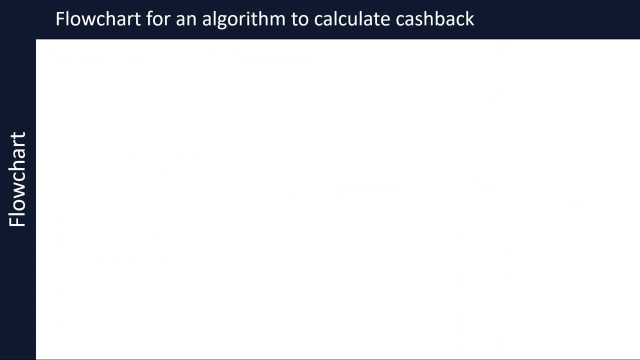 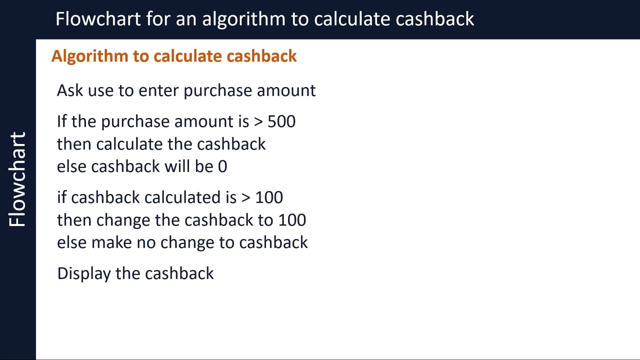 with the maximum cash back capped at £100.. So if the cash back amount is more than £100, then it is reduced back to £100.. Here are the steps of the algorithm to calculate the cash back. Algorithms allow users to enter the monthly purchase amount. 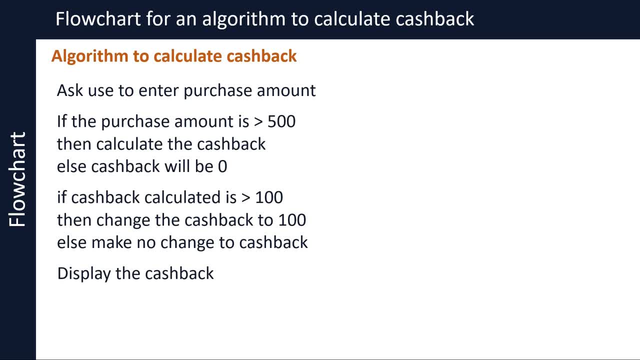 It then checks if the purchase amount is greater than £500, and if that is true, then it calculates. calculates 5% cashback. but if purchase amount is less than £500, then customer should not get any cashback, so cashback amount is set to zero. 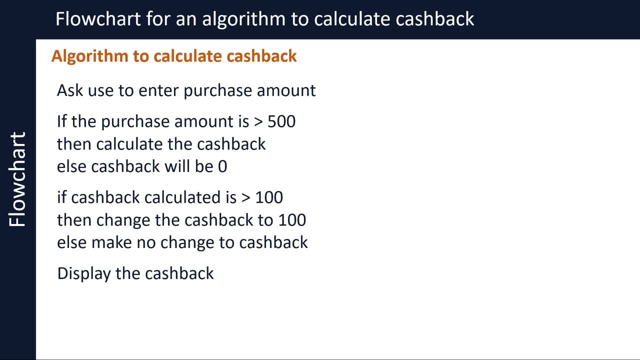 Algorithm then checks if the cashback is greater than £100, and if that is true, then it reduces the cashback to £100, but if cashback is equal to or less than £100, then it does not alter the cashback amount. 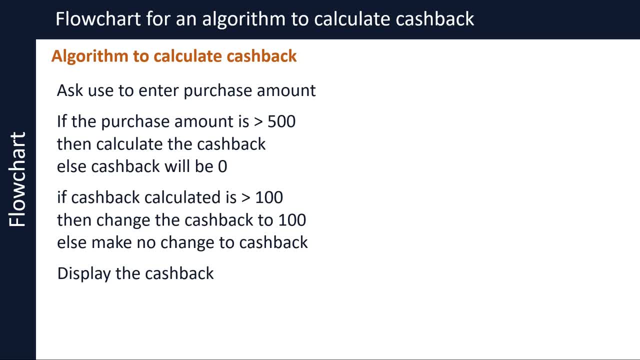 Finally, in the last step, algorithm outputs the cashback amount. Let's draw a flowchart for this algorithm. We draw the first symbol, as usual, to denote the start of the flowchart. Then we draw the next symbol to denote input where we ask user to enter the purchase amount. 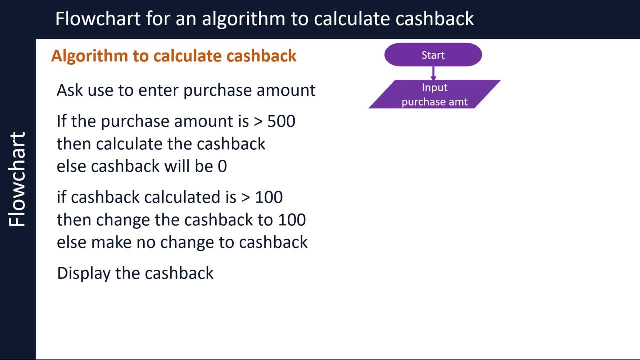 and store that into a variable named purchaseAMT. We now draw decision symbol to denote the start of the flowchart. Here we are checking if the value stored in variable named purchaseAMT is greater than £500.. We are using a relational operator to compare the purchase amount with £500. 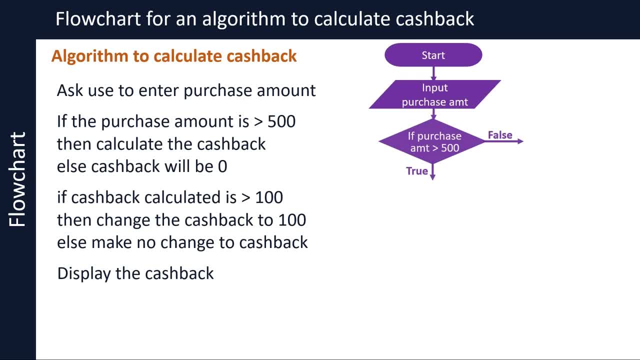 If the purchase amount is greater than £500, then we will follow the route along the path labelled true and calculate the 5% cashback by multiplying purchase amount by 5 and dividing it by 100.. We draw the process symbol to denote this. 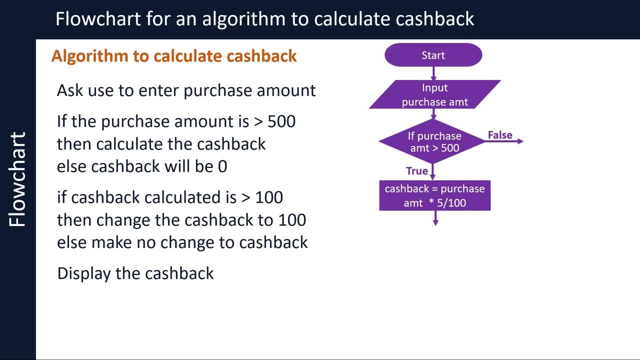 If the purchase amount is not greater than £500, then we will follow the route along the path labelled false and set the cashback to 0.. We draw the process symbol to denote this. In the next step, we again draw decision symbol to denote selection or decision. 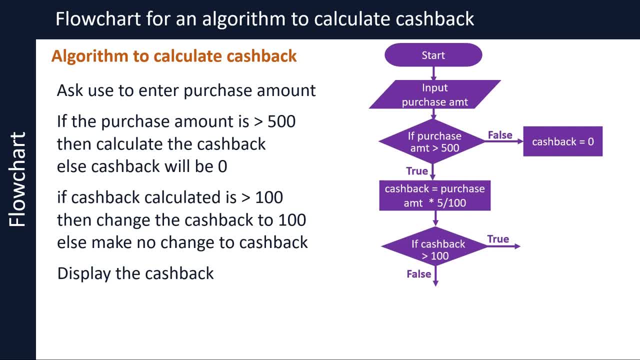 Here we are checking if the cashback amount calculated in the previous step is greater than £100.. We are again using relational operator greater than here to compare the cashback amount with £100.. If the cashback amount is greater than £100, then we will follow the route along the path. 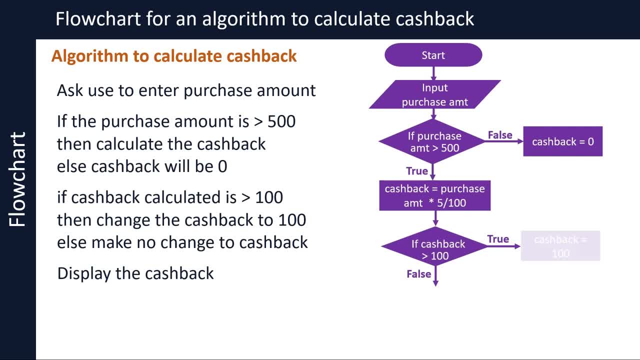 labelled true and set the cashback amount to 100. That is, we will reduce the cashback to £100, as it is not allowed to be more than £100. This is shown by the process symbol. If the cashback amount is not greater than £100, then we will draw decision symbol to. 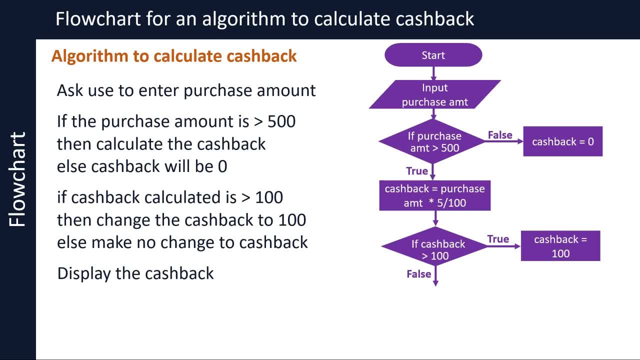 denote this. If the cashback amount calculated in the previous step diz double check, then we will follow the route along the path labelled false, or do nothing, or in other words, we do not change the calculated cashback amount Now, depending on which path the algorithm has taken based on the decisions taken in